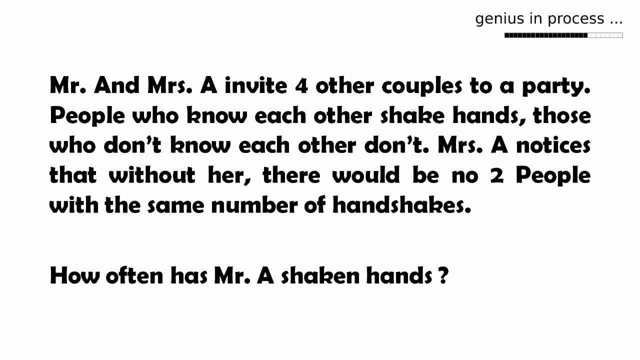 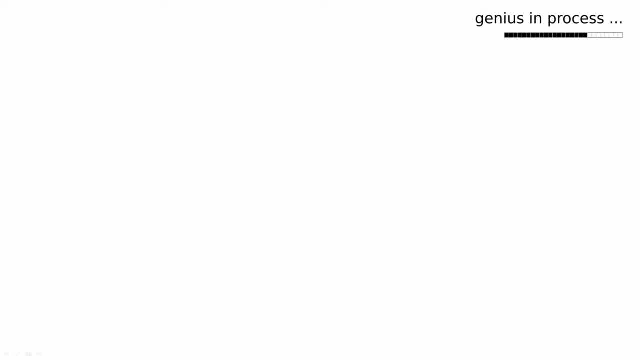 I've been very surprised that there is enough information to solve this problem when I saw it the first time, So I thought this could be a great challenge for you. Some general assumptions and observations to begin with. First, partners don't shake hands with each other. 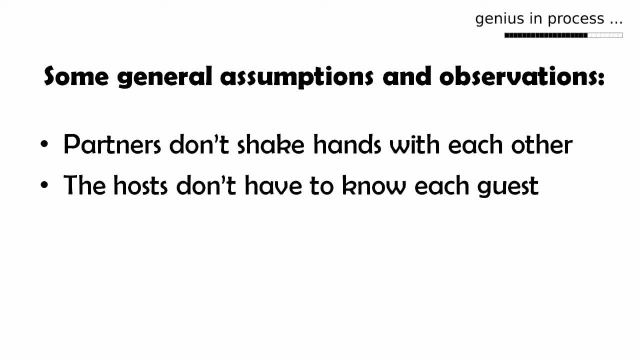 The second is the hosts don't have to know each other after guests. The maximum of handshakes is eight, because partners don't shake hands with each other, And there are nine people that shake hands a different number of times. Now how can we solve this problem? 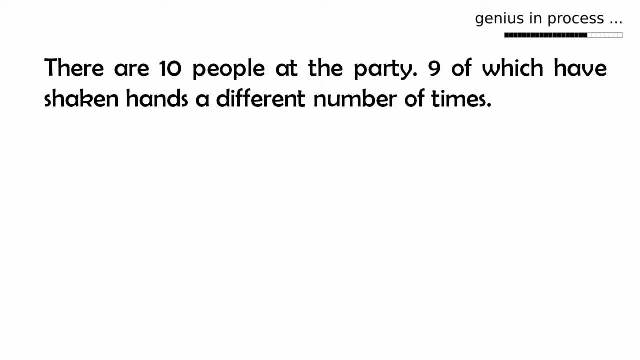 First of all, there are nine people that shake hands a different number of times. Now, how can we solve this problem? There are ten people at the party, nine of which have shaken hands a different number of times. The maximum of handshakes for one person is eight. 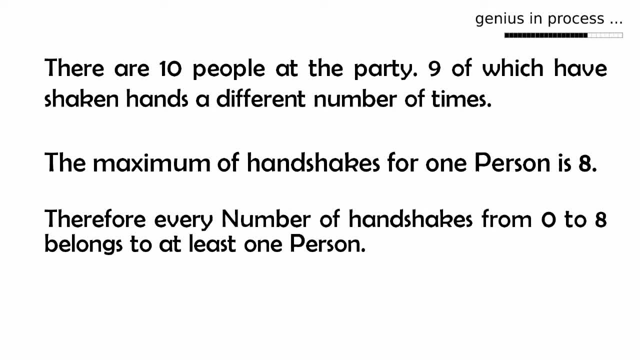 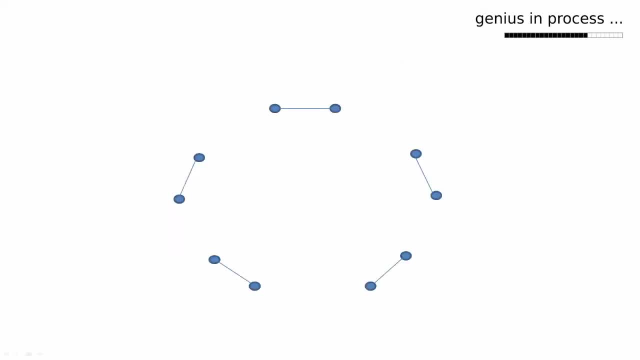 Therefore, every number of handshakes, from zero to eight, belongs to at least one person. To start, we visualize this problem by connecting every couple with a blue line. Notice how it is not clear so far which couple actually is Mr and Mrs A. 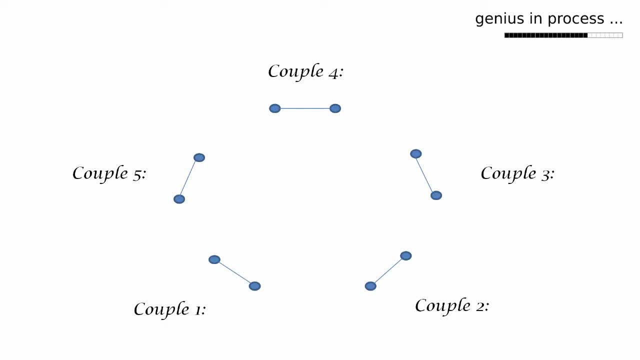 Because one person has to shake hands eight times, we can randomly choose one to do so. Now we evaluate how many handshakes took place so far, And we notice that the only one that can shake hands zero times has to be married to the one with eight handshakes. 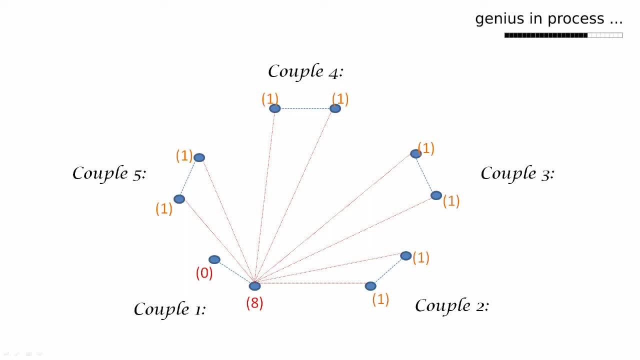 Now we can continue this process with the person with seven handshakes, And because everyone has shaken hands at least two times and the one with zero handshakes has to stay at zero, we know that the person with seven handshakes is married to the person with one handshake. 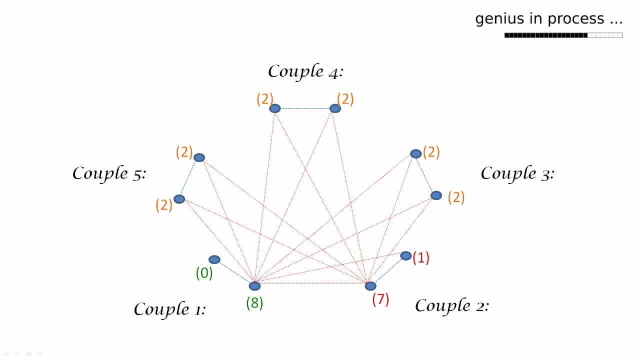 We can continue this for the couple which shakes hands six and two times, And for the couple with five and three handshakes as well. The graph we have obtained by logical conclusions so far contains every number of handshakes, from zero to eight so far. 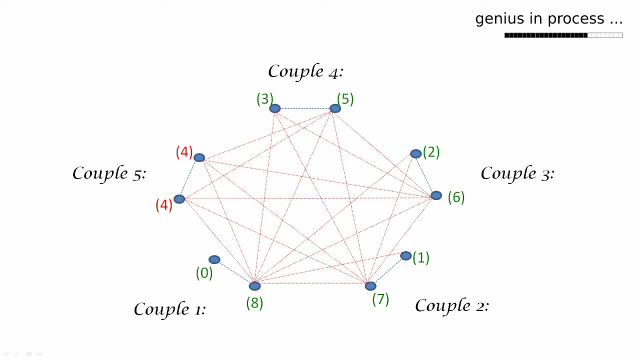 And cannot be modified anymore. You surely noticed that the last couple left has an equal number of handshakes and therefore must be Mr and Mrs A. In conclusion, because of exactly one couple with an equal number of handshakes for both partners.